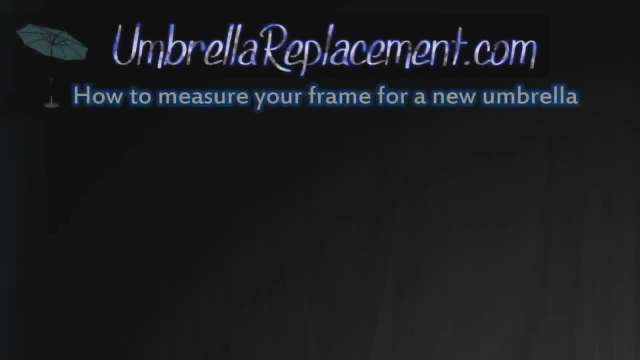 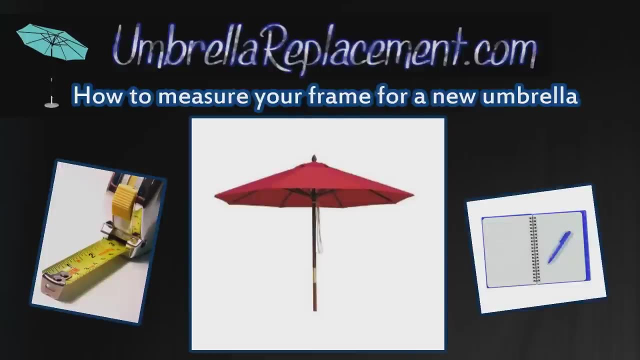 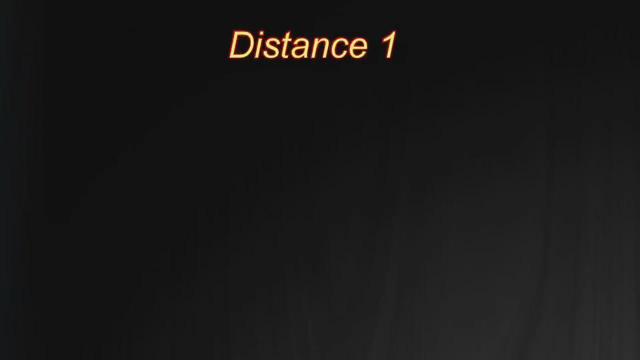 What we're going to do now is measure your old umbrella or Sunbrella so that we can replace it for you. You will need a tape measure, pen and paper ready as we measure your umbrella. We call this distance number one from one end of one of the rods or spars coming from the inside of the umbrella. 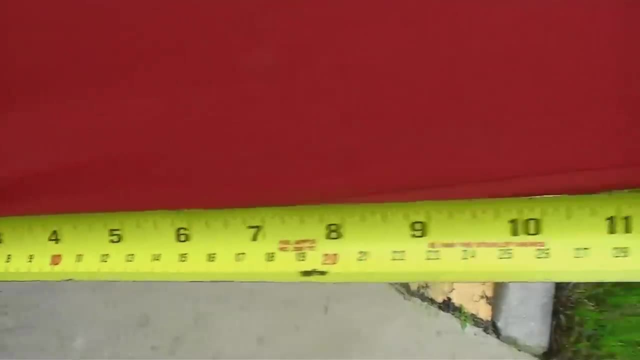 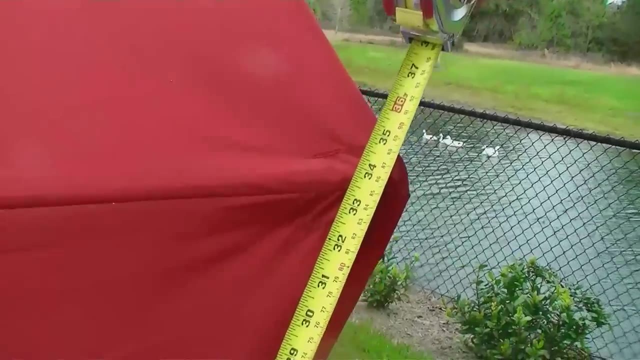 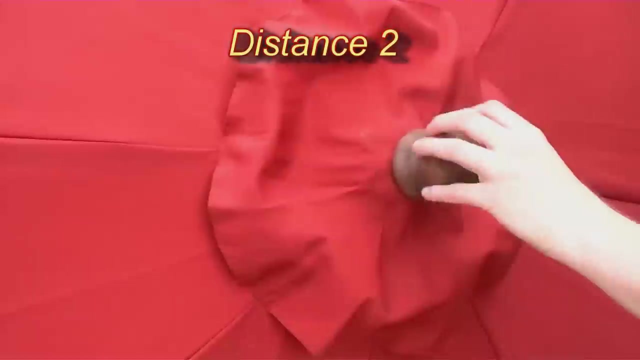 from the middle to the other, next spar, coming out of the umbrella and on here you can see it's about 34 inches. Be as accurate as you can: from end to end here. This is distance number two. You need to take this little piece off the top. 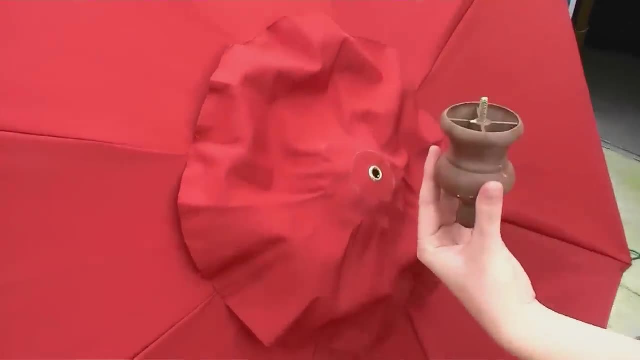 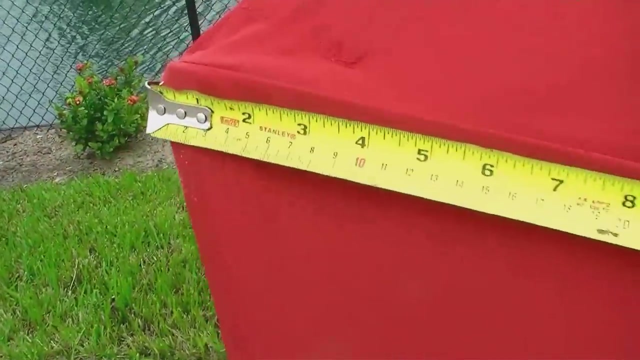 so that you can actually see the finial or the hole of the umbrella as shown. We measure this now from the end of one of these rods, right from the very tip, as you can see here, right to the middle. This is the middle of the little hole at the top of the umbrella. 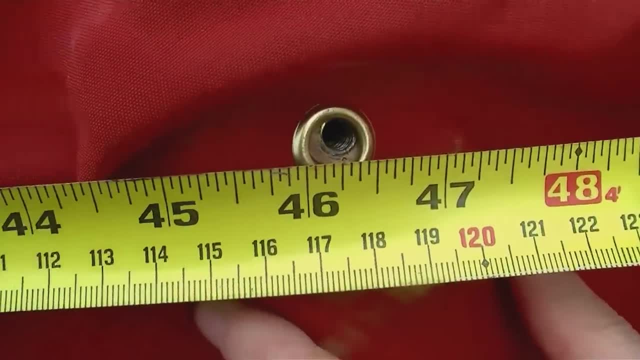 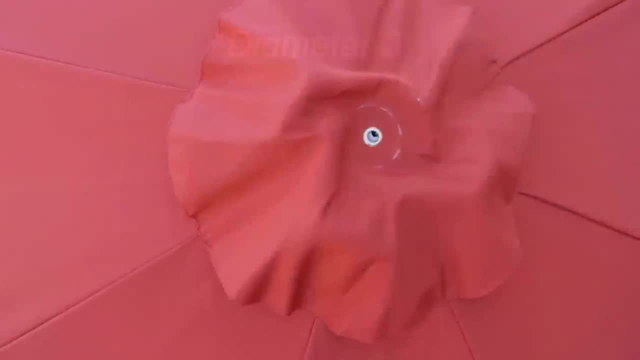 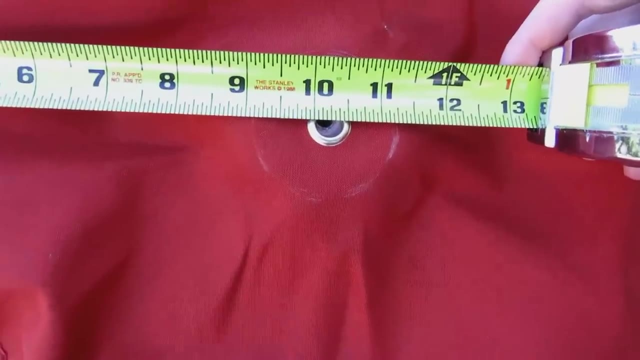 So this is about 46 and a quarter inches on this distance. Now we're going to measure diameter number three. This is the diameter of this little hole here. As you can see, it's about half an inch across the diameter of this little hole. 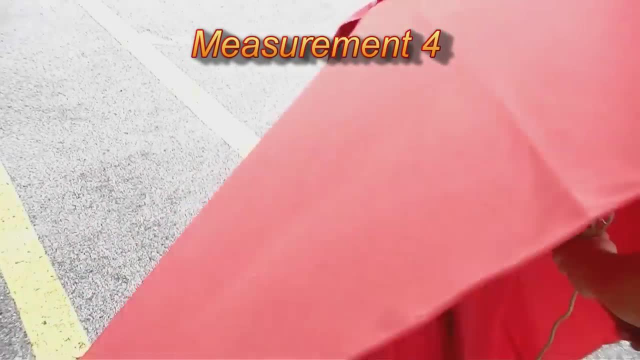 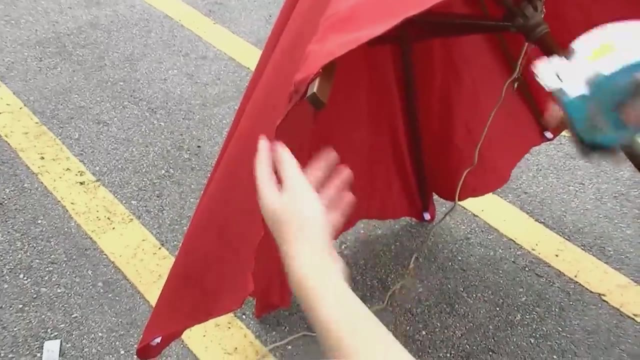 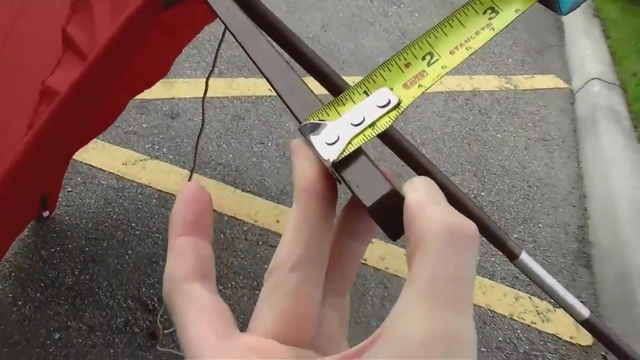 This is going to be measurement number four, which is very important. We're going to measure one of these spars or struts, and we're going to measure the width and the height of this strut. This distance across here is just under seven sixteenths of an inch. 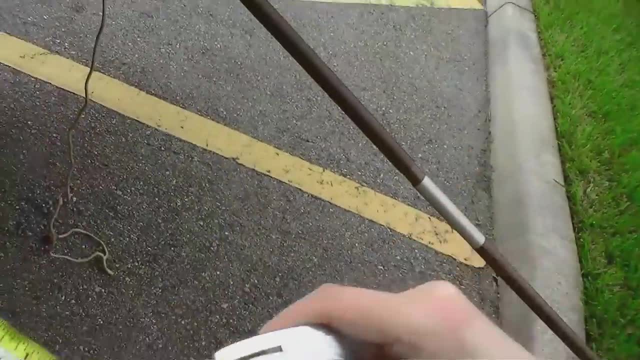 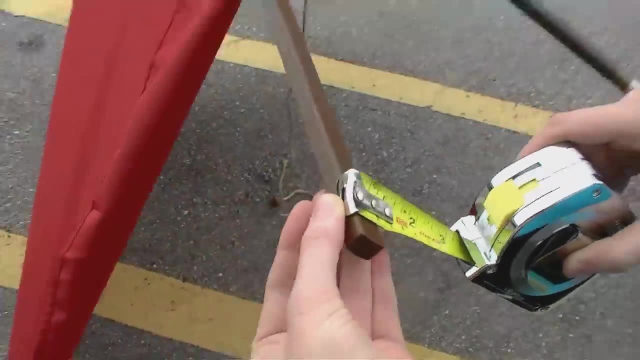 You need to get it as accurate as possible And also we need to see, as you can see here- measure the height accurately as possible, and that's about three quarters of an inch, As you can see on this umbrella, which is a sample that we have just to show you. 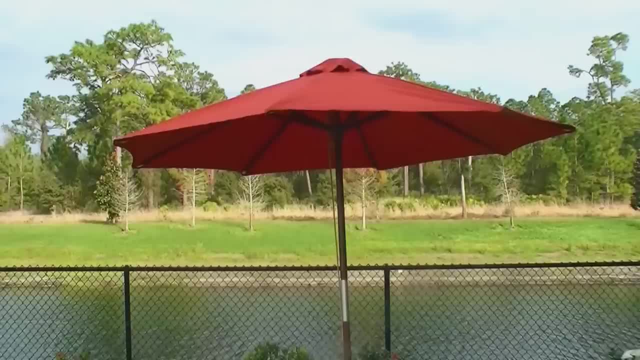 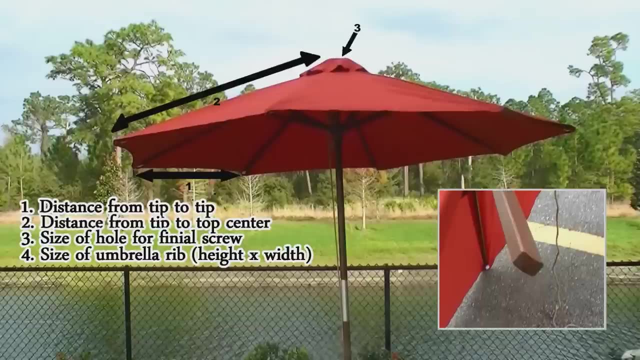 you can see the dimensions and the distances that we require: Distance one, two, three and then the final one is the strut. We need that. That is very important: the dimensions from the width and the height of that little wooden strut.